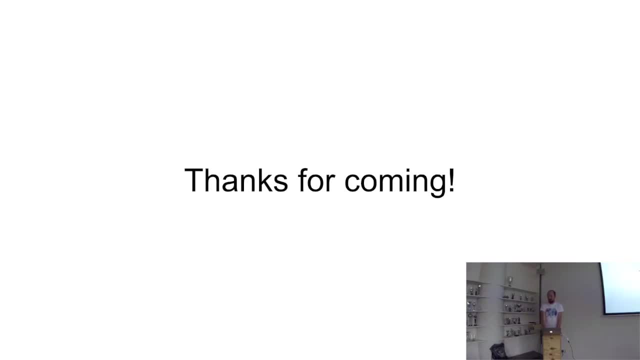 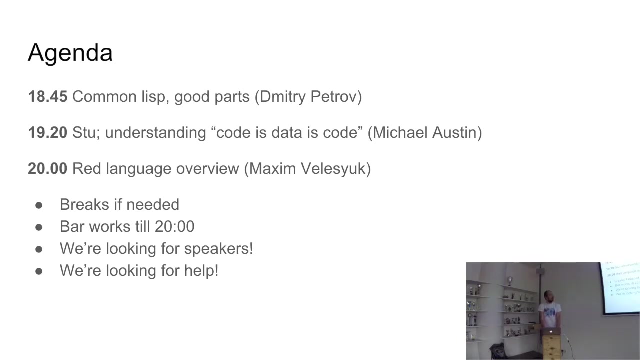 Hey everyone and thanks for coming. It's actually quite surprising that we got more than us in this video. Let me quickly go through the agenda, So I'll be the first one talking. I'll talk a bit about comma list And then Michael will talk about stu, the list dialog that he develops. 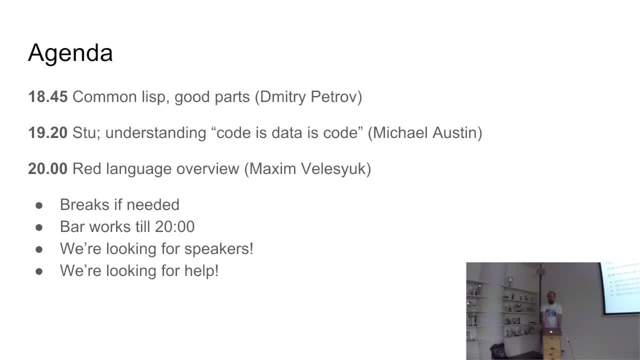 And the last talk will be from Maxim about red language. that shares a lot of features with list, And probably even more list than list, So we can make breaks if needed between talks, And it seems like we have no problems with drinks, of course. 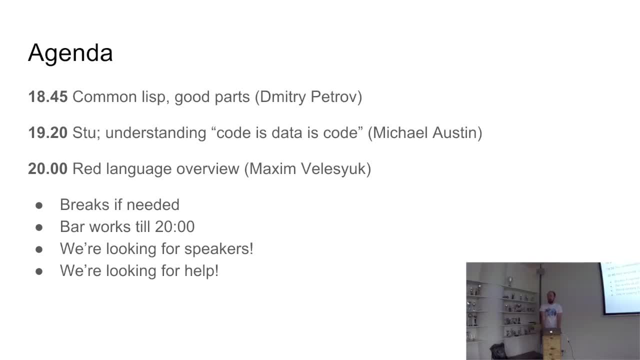 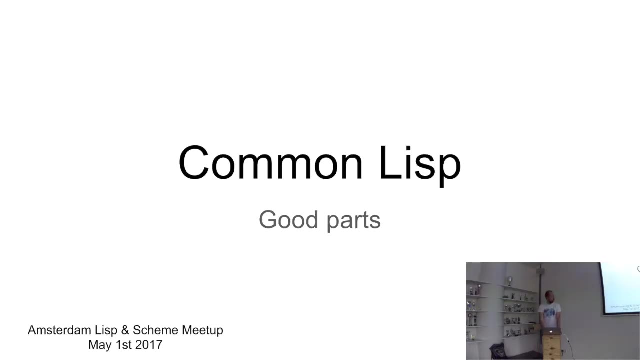 The bar is not necessary, But if you want to talk on the next meetup, just let me know, And if you want to help with anything like location next time, also, please contact me. So my talk will be about comma list and how many people actually used comma list. 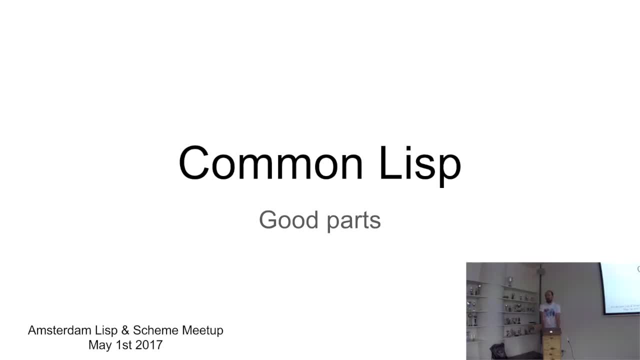 Okay, At least some people didn't, And that's nice. Yeah, So it will be more experienced report for me, because I'm not a pro comma list developer. It's more like a feature that I find really fascinating when developing and compared to mainstream languages that I use on my daily work, for example. 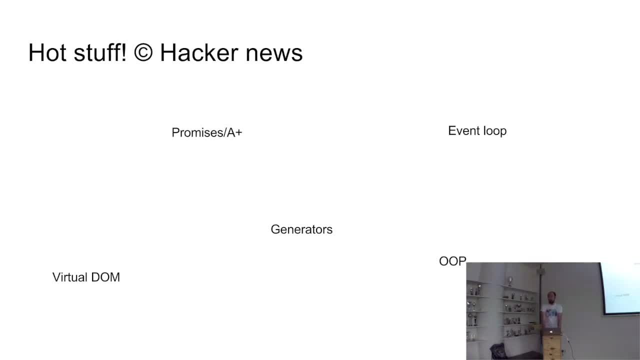 And yeah, when you don't have like really good computer science background, then it's really easy to lose the sight of technologies that were developed a while ago. So you check out Hacker News And, for example, if you use JS, right, what you see like, oh, we have promises. or, like you know, event loop generators, virtual DOM. 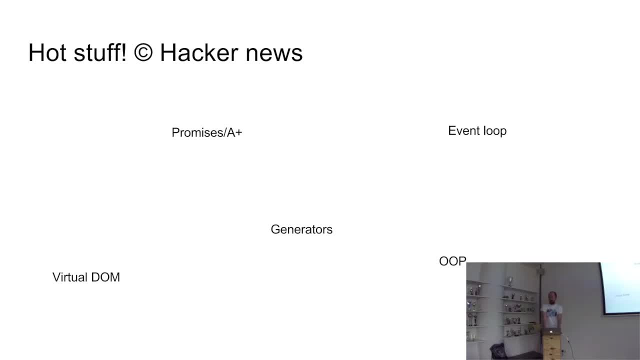 And you think of it. it's all new And well, it wasn't there before, right, And this is how you imagine the world, right? It was like from a middle ages where there was nothing- mainframe cards- And then we are in the bright future where we have fascinating languages to work with. 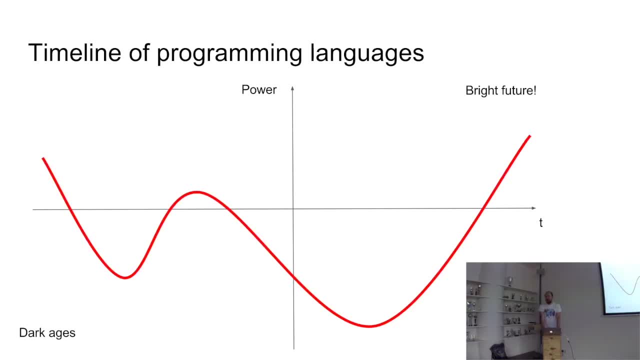 But, to be honest, it's more like this, right, It's like whatever language catches the hype and maybe has a big corporation behind it, And the one is the one that gets the majority and gets a lot of developers. So for me, it was mostly like this: 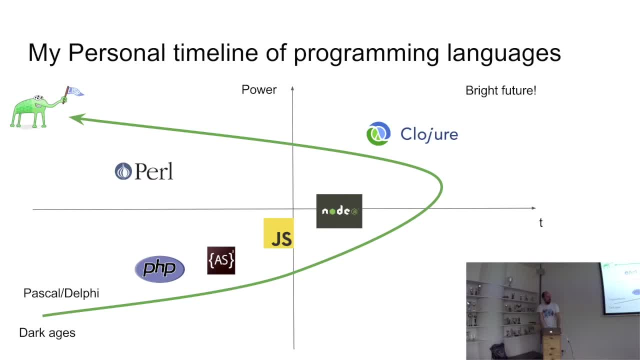 And so I started off with Pascal and then moved to web development, And at some point there there was a turning point where I read Interaction to Closure, And I read one more, a few more books And I thought that you know, like the life will never be the same again. 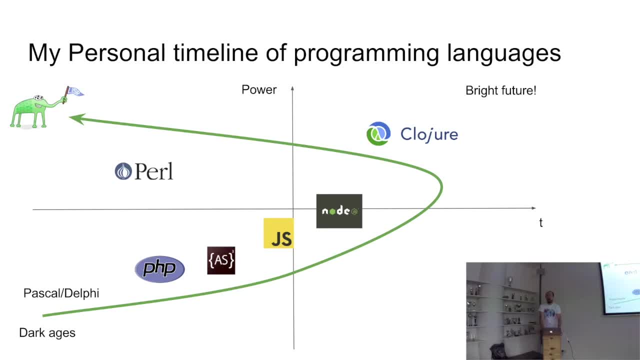 Because it really has a lot of stuff about interactive development, about immutability, And it really makes sense right, Especially if you return back to usual languages after that And so like, why would you ever do this if you can't do like that right? 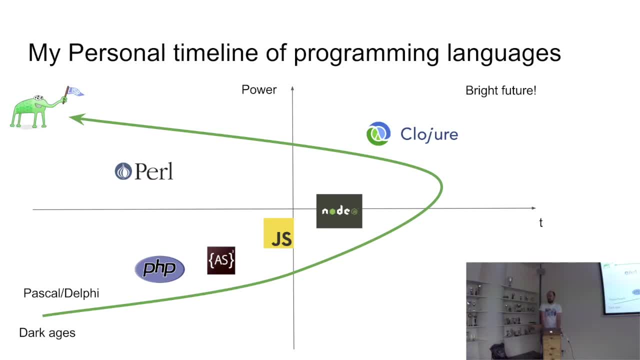 But if you really like the language, you try to do everything with it, And it was my case. So I decided: okay, I want to build all my command line tools with Closure and all the rest, And it seems like. it seems like Java is not that awesome for command line tools. 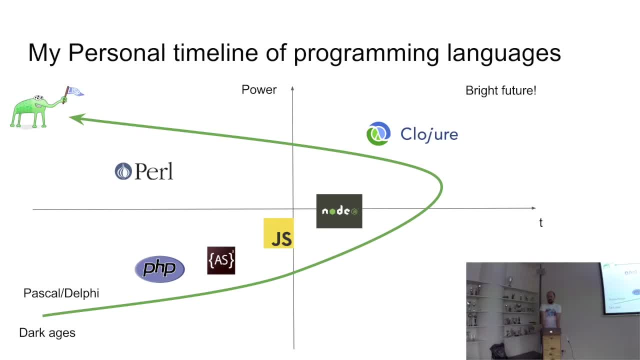 Especially if you want to make them fast enough, Right? So startup time really matters, Not for web development but for everything else. So and I had a bit of you know like complex that I, all the discussion around Closure, had a thread where people say like 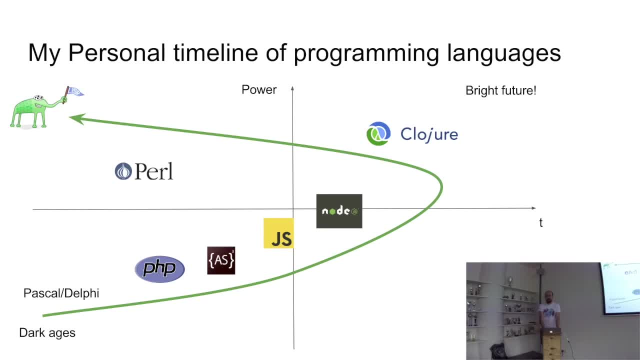 no, no, no, no. check out Common Lisp. you know, like Lisp 2, Lisp 1.. It's not really Lisp and all this. So I decided to go to roots and check out Common Lisp and see what's actually there. 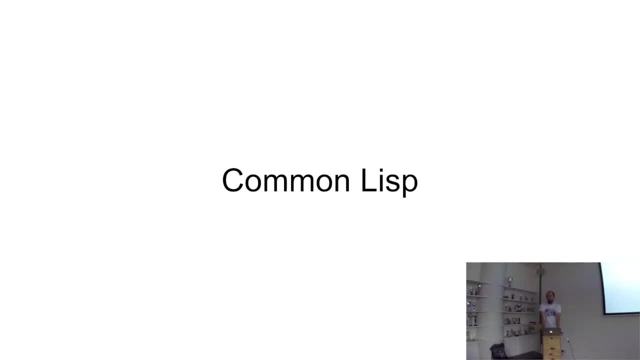 And there are. there are bad parts, for sure, there, And most some of them are a reason for decline in the popularity and all this. But there are exceptional parts that makes the language really different And these features are so powerful that I well that. this is why I tried. I write all my hobby projects with this language. 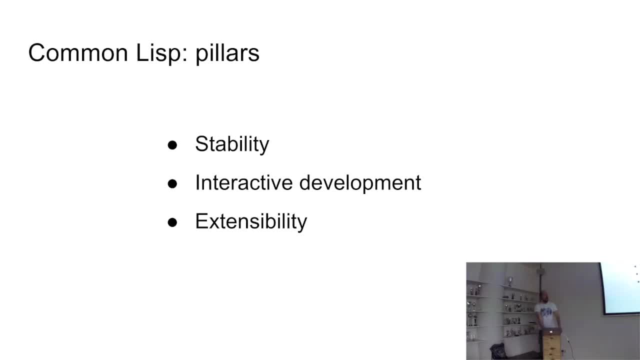 So, for I think the main three points are stability and interactive development and extensibility. So stability is an interesting one, because if you compare Common Lisp to any other language currently used, they are all not- how would you call it Not that stable? because, well, not every language has a standard that is like 20 years old. 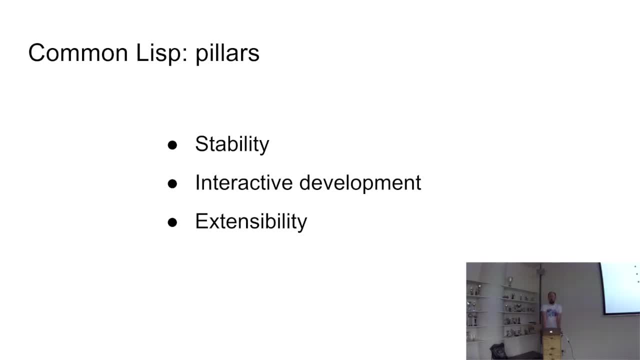 Right And have a bunch of compilers that are in active development that support it to a very good extent And, as we discussed earlier, that you can just take the code that was that was developed years ago and you can write it. write it on a modern, modern compiler and have it working. 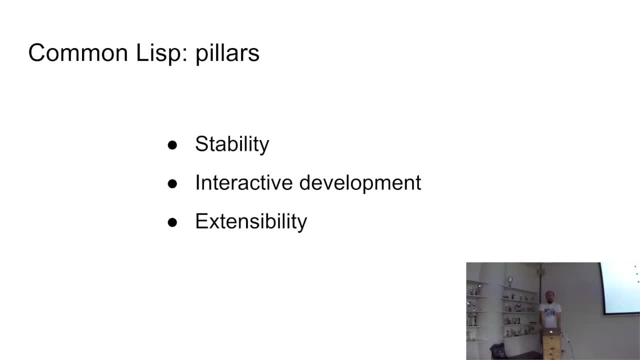 And it's amazing, Especially to younger ecosystems, where you, you know, you return to a language like two years later and nothing worse. Everything is different. You're like: oh no, no, Like, where are my libraries? So second part is interactive development. 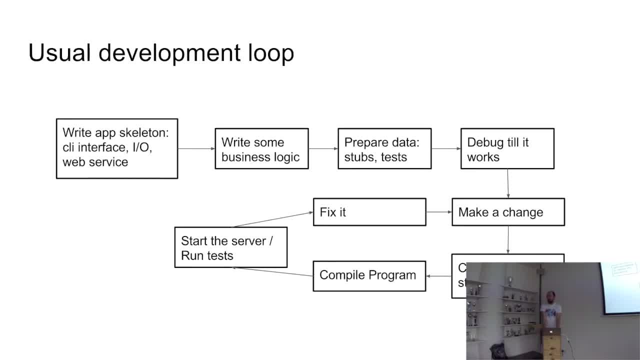 I don't know if I need to promote it a lot, but I'll have a couple of words, Of course. So this is a usual loop, how it works with like languages like Perl, Java and the rest. Right. So you decide to write a program and then you're like: okay, so I need to do some business logic. 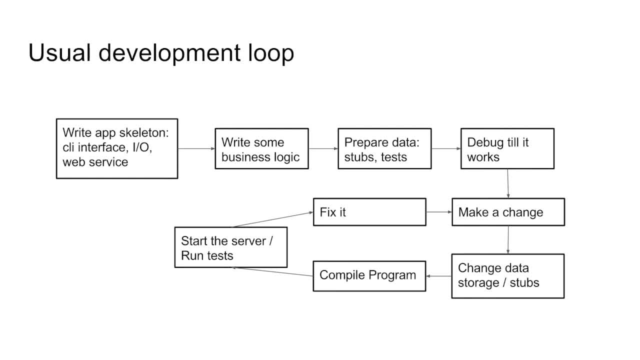 What should I do for it? Okay, You need a skeleton for application because you need a common light interface, You need to feed it some data And you write all of this and you spend like 20 minutes if you're lucky. or you can spend a couple of days if you have some protobuf protocol to store the data or have tabs. 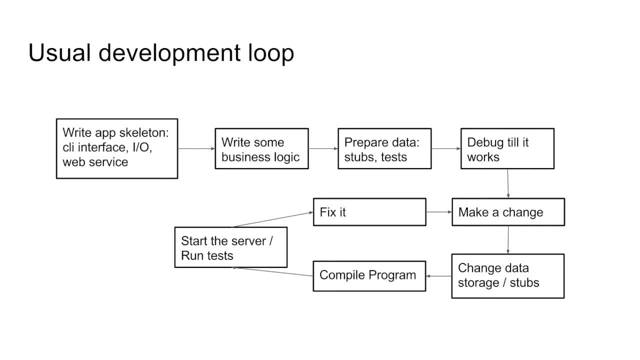 So, and when you write this pile of code after you say like now I am totally ready to write some business logic, right, And you write it, and then you need to update all the rest that you already wrote, And then you need to add some code that you don't want to add to to update state. 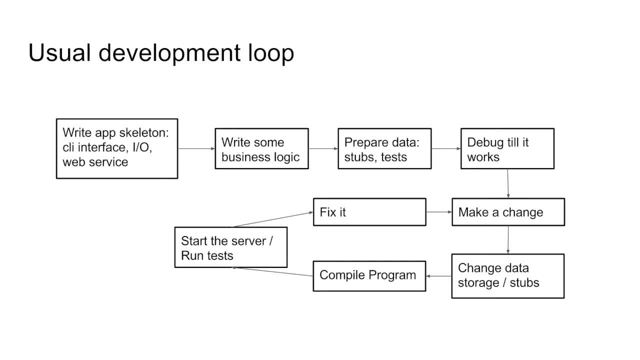 And you compile the whole program, run, hope it works, do it again. And this loop is quite large. For example, in booking we have big systems and restarting the system can take a couple of minutes Right, And that means that you can restart it and find out at the end that you've made a syntax mistake or runtime error that you could catch much quicker if you could just compile this little piece of code. 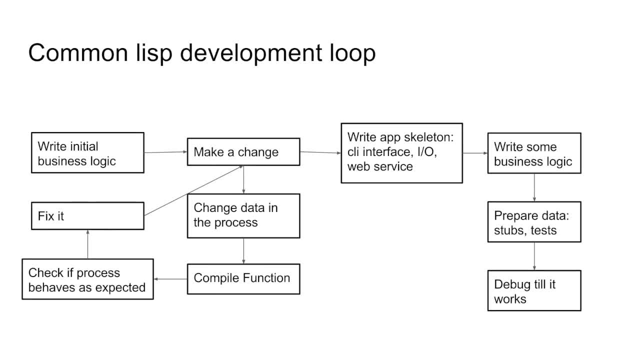 Right, And this is how CommonList works. So right here you can start the process and write initial project. right there You define functions, you work with it, you can generate, stop data on the fly And you see if it works. 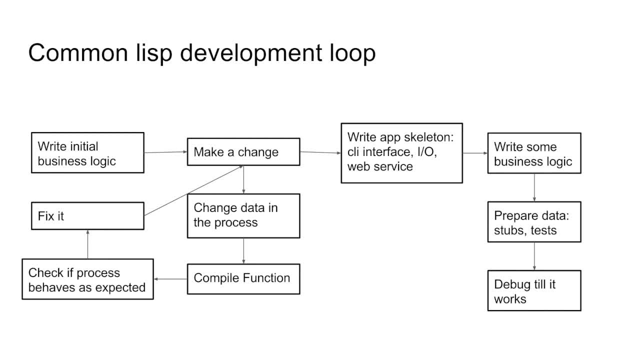 and you can compile individual functions and make it working. And it's really easy to get some prototype in a couple of hours because all you need is to business logic to write, And this process is shared between Clojure and CommonList And in many cases this loop is all you need. 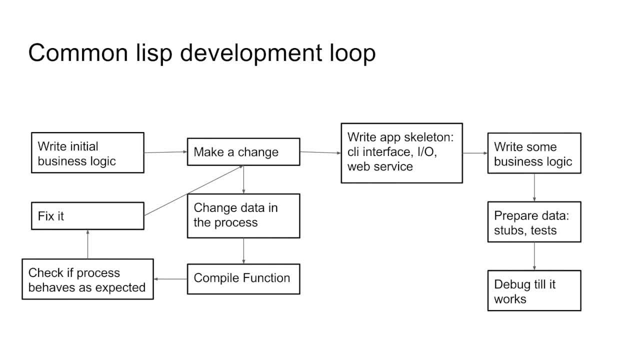 because you just need to write this business logic and test if it works, for example. right, If it works, then you're done. For example, you need to produce some data or some numbers, And only if you need to put this code in production. 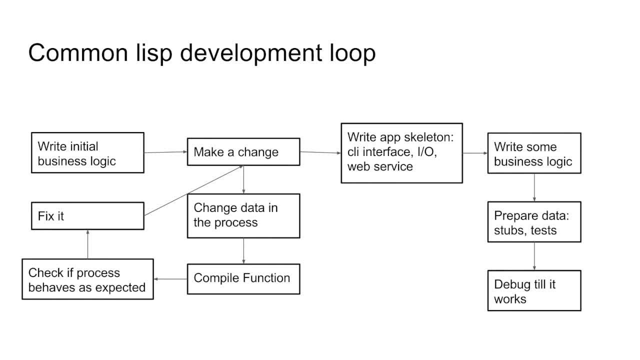 or to make it. you need to share it with someone And you can write to call like interface or web server. but it's all done afterwards And, of course, after you write all the rest, you will get this bigger loop of changes. 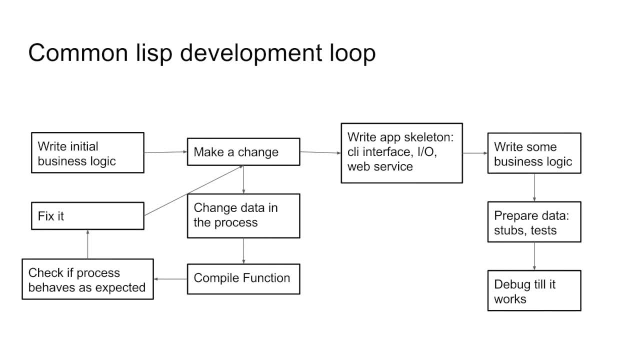 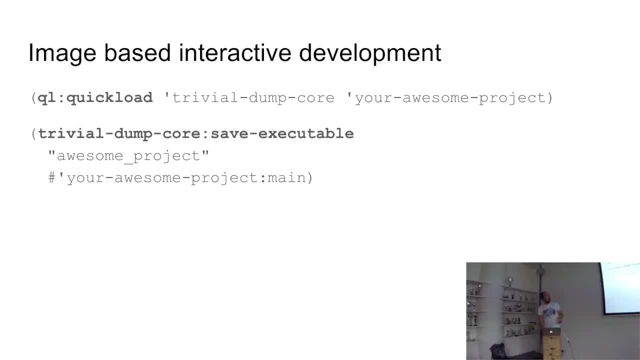 But still you can get much quicker changes because you can recompile individual parts and have it working right there, And this is in ListView. this is mostly possible due to image based interactive development right Where. so, with difference of- by the way, these are not official terms. 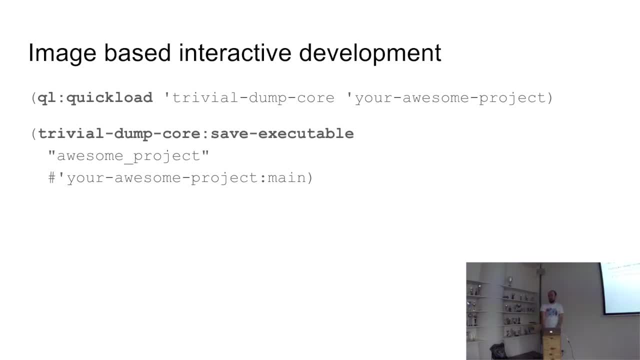 So if I'm like playing wrong in some terms, just correct me please. Yeah, So in the ListView you just start the process and you load the libraries and you work with them, right, And everything is transparent. So you can inspect every part of your code. 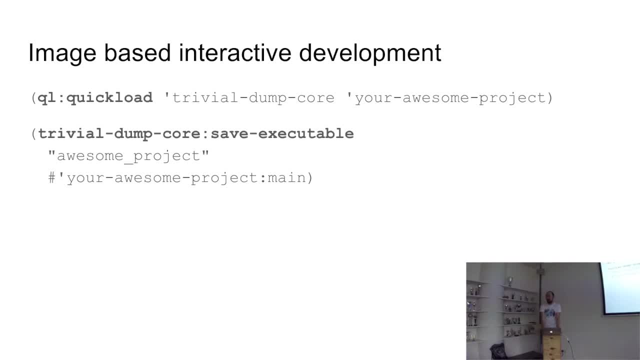 And this is a very big difference to other languages. And this is, for example, my personal road, one of my personal roadblocks, because you're like you write your code in a REPL and you're fine with it And then like: okay, how would I compile it? 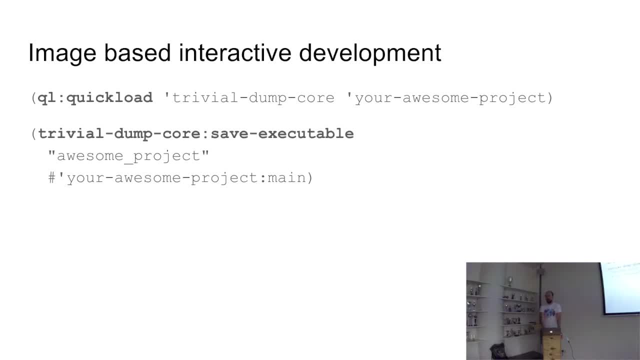 And you go like compile, compile. but there is no such thing as GCC, where you parse the source right And the whole compilation happens when you load your libraries in the process and then you dump the image. So, and the different- and this is a difference- with Clojure. 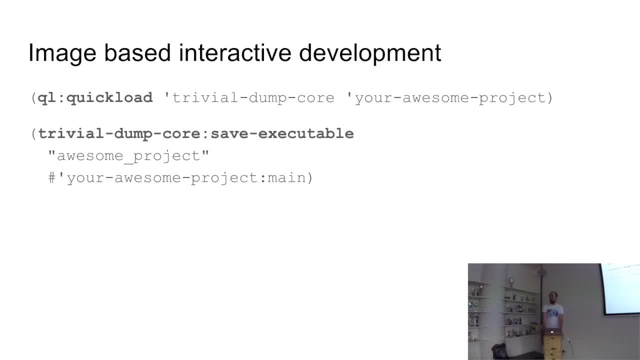 because in Clojure you actually build an application right, You get the bytecode and here you save the image, And this image contains compiler and all the all the development environment And well, the startup time are really fast. So if you write your command line tools, 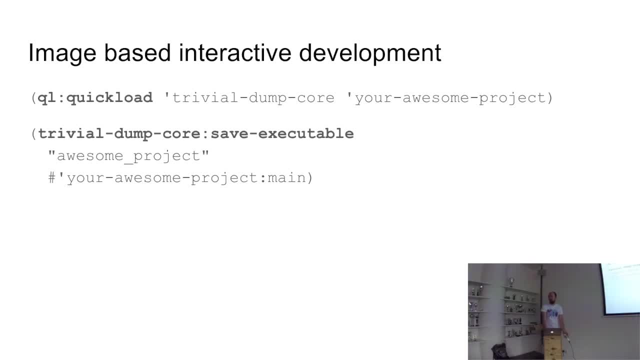 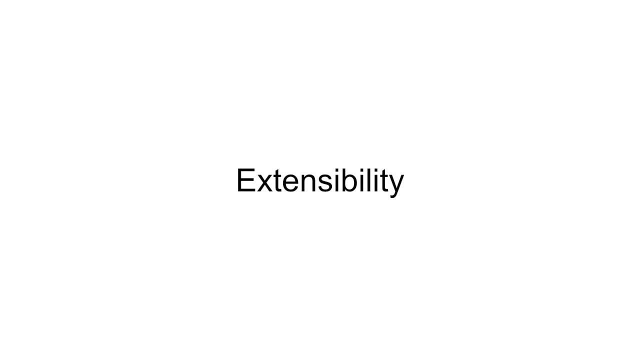 they will start in 30 milliseconds or something like that, Which is which really makes much more sense for me. So the last point is extensibility, And there are many parts with it. First of all. first I want to highlight is just to showcase for extensibility in Lisp right. 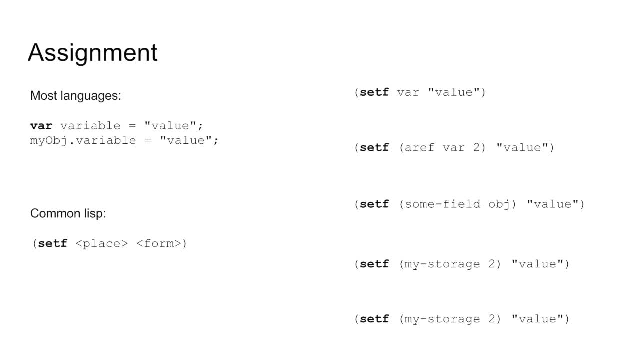 In many languages the assignment is like this: You have variable right, You're sending some value And if you have an object, you can assign. you know, if you have an object, you can assign some value, And if you have an object, you can assign some value. 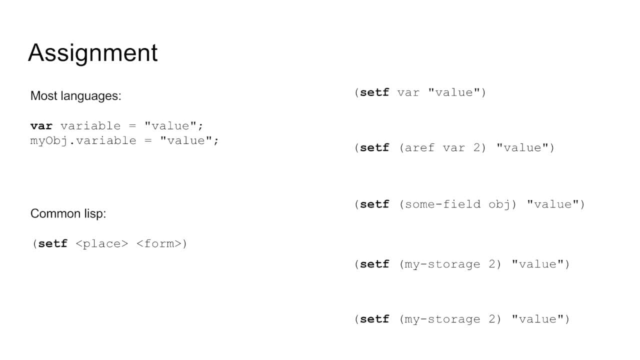 And if you have an object, you can assign some value. And if you have an object, you can assign some property to a field in this object. And well, maybe you have a setter for this object And this is all you have for extensibility. 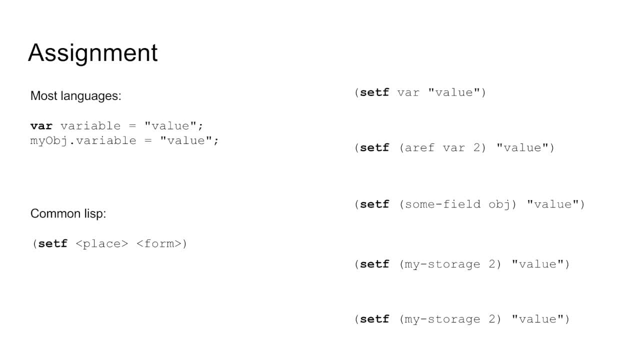 In the common Lisp there is a set of operator that operates with the notion of place and form right. It evaluates a form and puts it in a place, And this place, if you take a definition of place and the variable, is just one of these two. 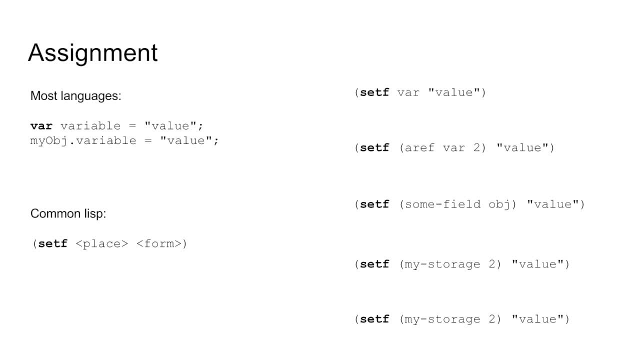 And the variable is just one of these two, So you can assign the variable. But, for example, a function code can be a place or any accessors to the common Lisp to the slots can be defined as place right to the slots can be defined as place right. 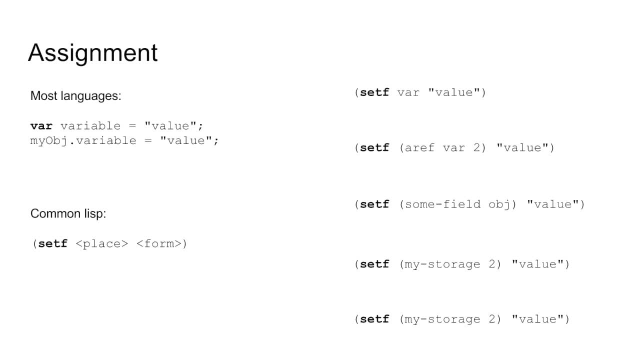 And, what's more, you can define your own function that will work as place, or you can define a completely custom form, customized form that will work like this And that makes it adds another layer of abstraction where you can place your logic. that will be impossible. 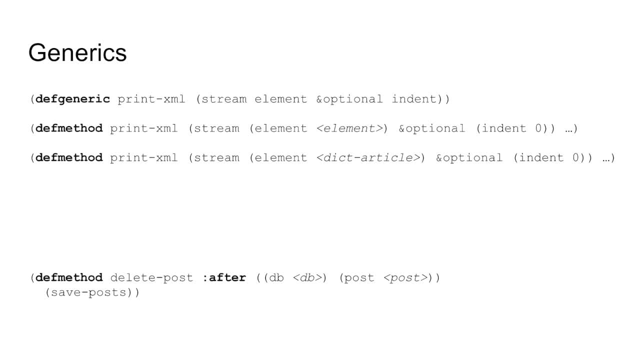 in the cases like a plain assignment. Another and yeah, another cool thing in common: Lisp is generics, and well, the way it works if it is, you define a generic with signature and then you write an implementation of it and you decide. 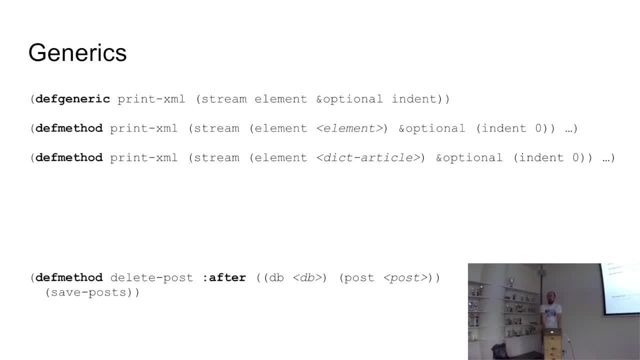 and then you write an implementation of it and you decide you can dispatch it against certain types of arguments, And the beauty of it is that you don't need to dispatch it against one type, as you do it in JavaScript, for example. You have a method on object, you call it. 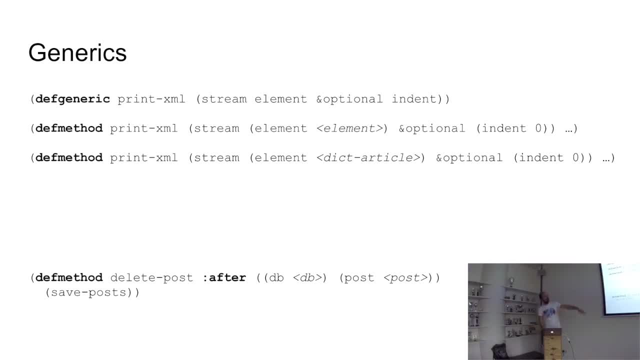 and it has this value And this is where you use for dispatch. Here you can dispatch against all the arguments, And the fact that it is take it away from the object, take it away from the object definition makes it really powerful in sense that 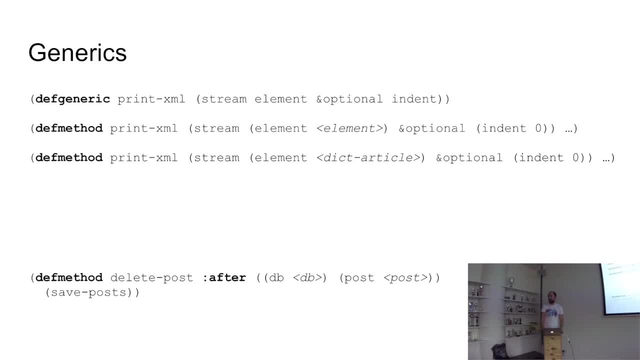 you don't need to extend object right. You can write a function definition. you just put it on any object that you can. You can take a readily available external library and if you can take object signature, you can already write new functionality on top of it. 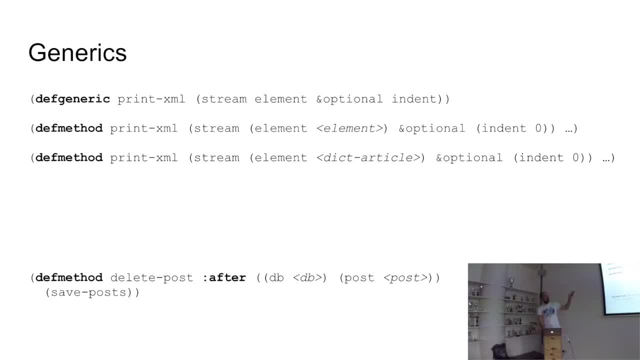 and you don't need to inherit from objects. For example, you have a DOM tree and you want to print it your own unique way. You can define generic and then define concrete types that will print a function in the way you want. The other extension point: that is really awesome. 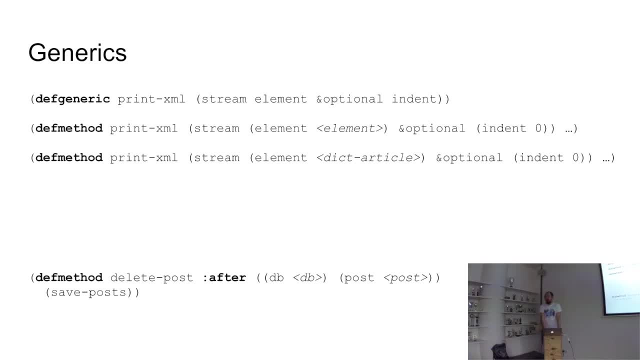 is that generic, support aspect-oriented programming. and that brings yet another extension point. For example, your library can define certain operation and generic functions and then you don't need to override this function, or you don't need to override this function, or something. 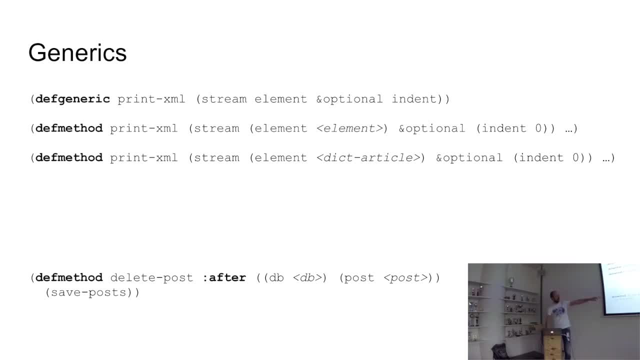 You can just say okay when delete post function happens in that library. after that, I want to well do some IO, for example, And you don't need to couple these. It will be right there in your code. And yeah, the last bit is objects. 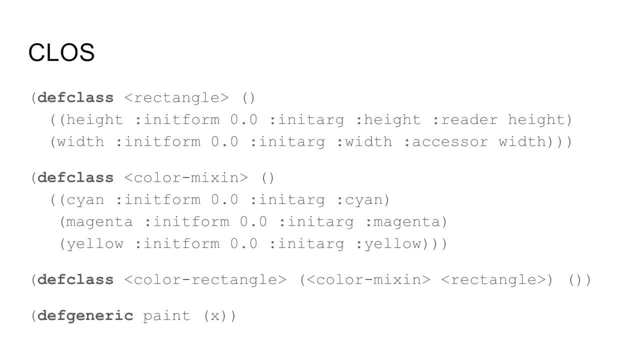 and the coolest feature of it is that once you detach a method from objects, you really have much less problems with multiple inheritance, for example. right, You have only slots. You don't have collisions in methods or in signature of these methods. It's just, and that makes it really simple to define. 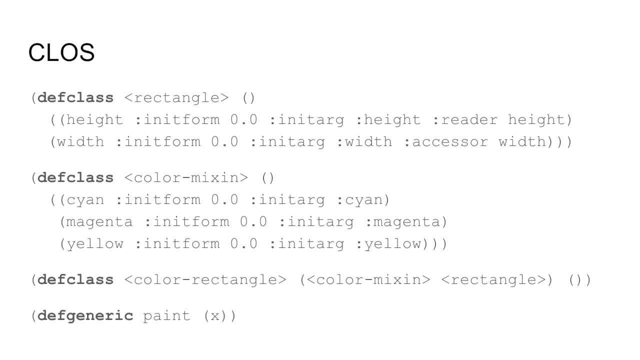 for example, classes like color rectangle, which has two mixins that are just backup properties and then you can have a generic paint right And then, for example, with aspect-oriented programming, you can dispatch against color rectangle and set up all the color facilities. 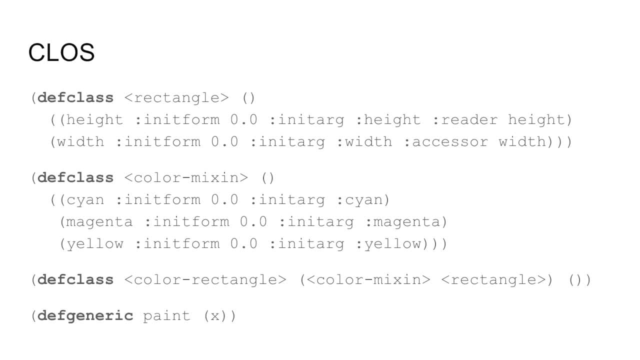 and then you can render rectangle with other code and it will be totally decoupled, and yeah, and you can, for example, produce all other shapes. So this makes it easy, really easy, to decouple functionality. Yeah and yeah. the last bit is macros. 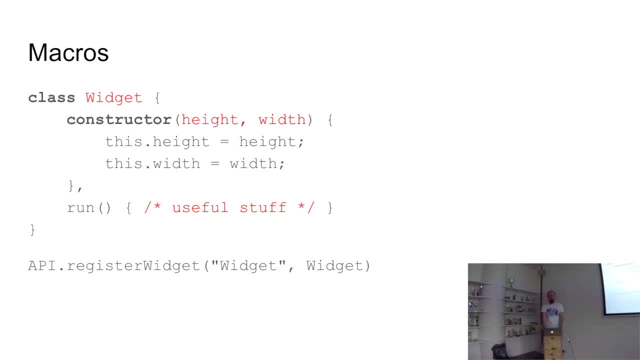 So in usual C-like languages, for example, you want to define a widget right, And you write the boilerplate code and you might be asked like okay, so where is the duplication? And you say, like there is none right. 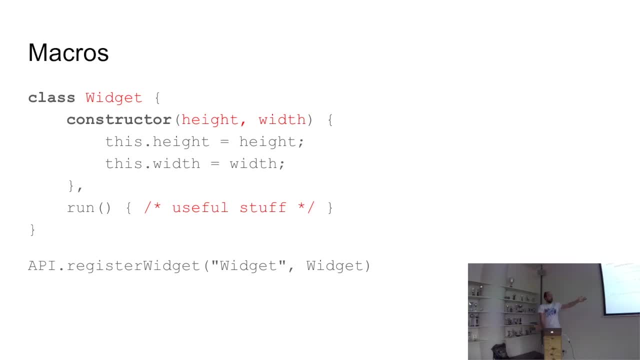 It's just like I need to write a class definition and the fact is that if we look at it from a common list perspective, it's just only those red parts are unique. All the rest is duplication, right. You just write the same class for a constructor. 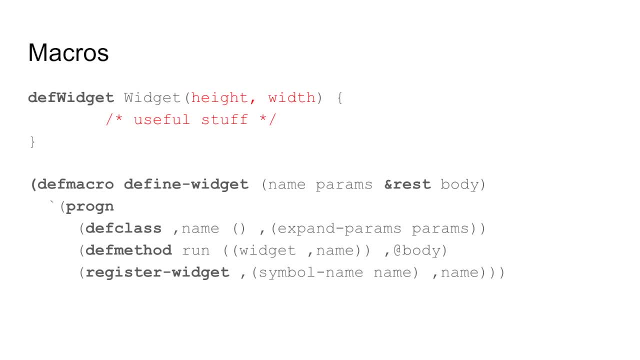 all the rest. Wouldn't it be nice just to say def widget, define parameters and write stuff, and this is what macros allow to do: to find new control structures and to hide some compile time, some things that could be done compile time. 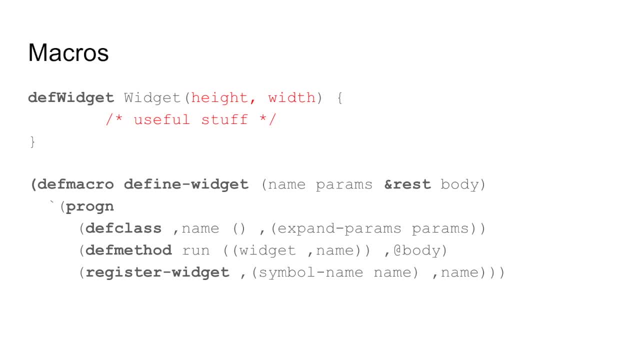 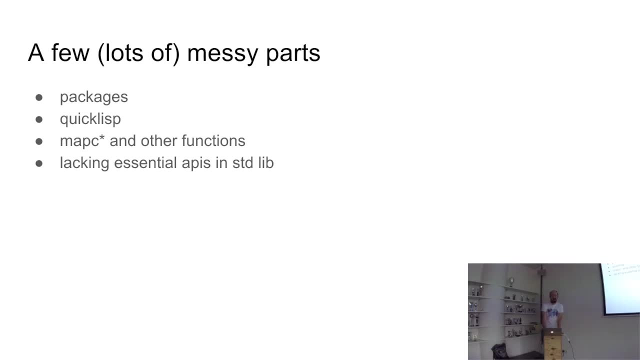 or define or remove boilerplate code that makes your code really dense. Yeah, so this was good parts and these are a couple of major parts. So, since the language is that old- the fact that the last release of library is five years old, for example- 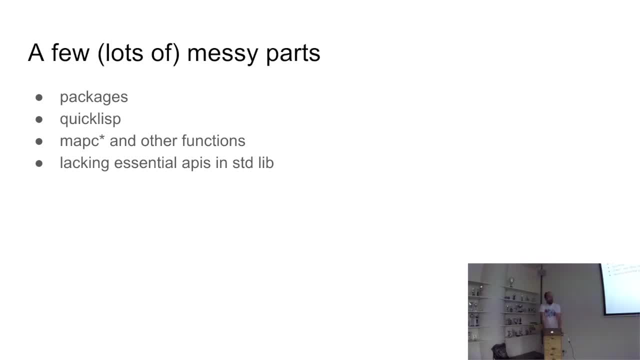 doesn't mean anything. It's like fresh, new or at least not that old right, And a lot of really, really, really, really, really, really popular libraries on the common list standards have some problems with documentation, for example. 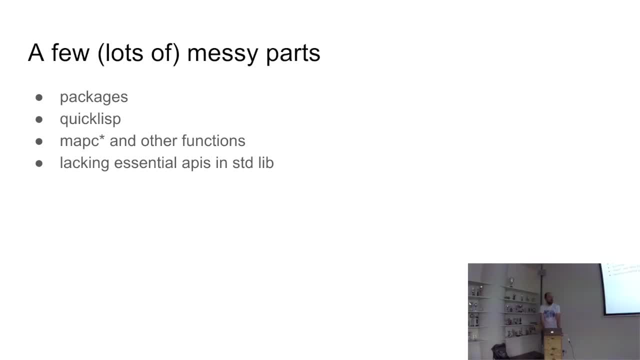 or it's written not in a nice way, So, and QuickLisp is a relatively recent improvement, right, So for a long time in terms of common list history, they just say like: okay, just download your system. 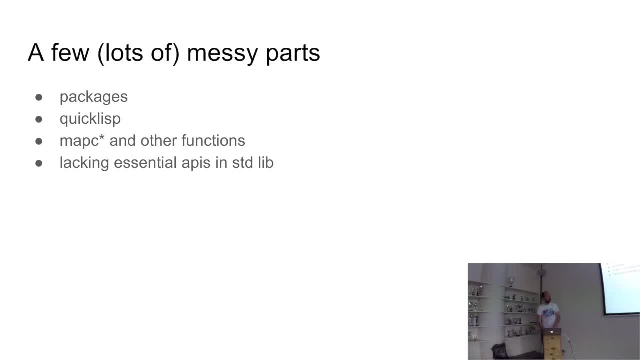 you place them somewhere, you load them right And it was a pain point. And yeah, Since language was built as a unifying platform for all the dialects, of course it has some features that are not coherent or like not as nicely built as enclosure, for example. 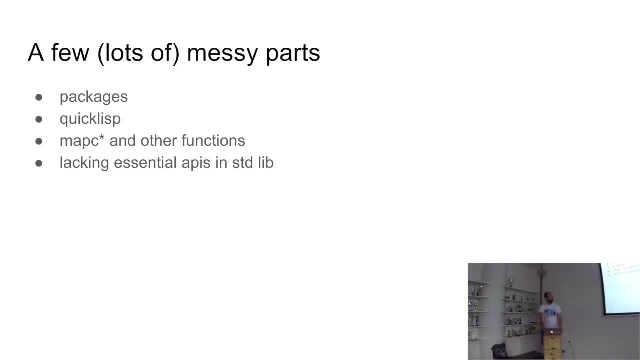 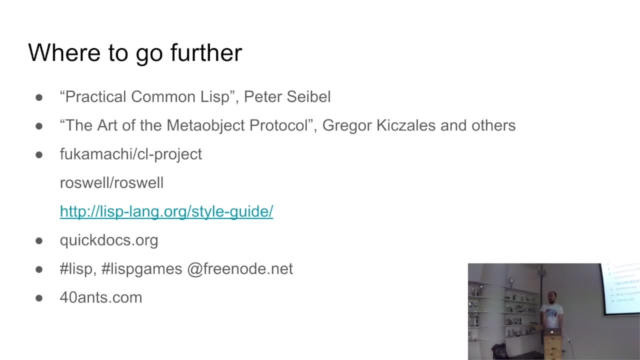 But yeah, it's what we have to live with. And yeah, as a conclusion, if you never, if you never tried OutLisp, but want to just read about language, I think the best book ever written is Practical Common Lisp. 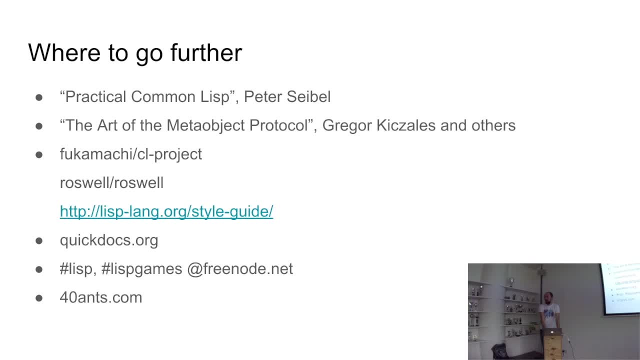 I use it as a reference all the time and whenever you want to understand, like why things work the way they work. most probably in Practical Common Lisp you'll find a good explanation for it And it's available online. If you want to understand how the Common Lisp object system works. I think the other great book is The Art of Meta-Object Protocol, because it really defines all the reasons why it was done in the same way, in the way it works, In the way it was done and why it even features. 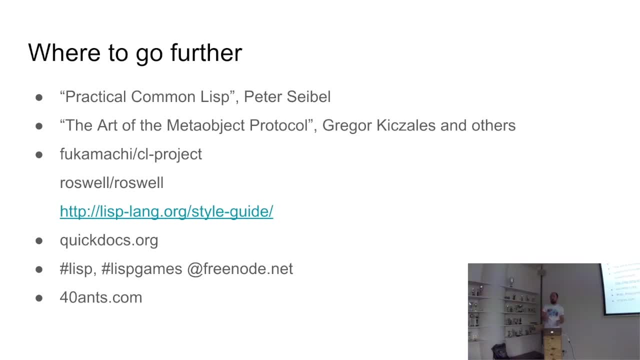 the implementation of simplified Common Lisp object system. So they discuss: okay, this is why we do this or this is how we do inheritance And the rest are links. So these are GitHub projects. if you want to quickly bootstrap a project, 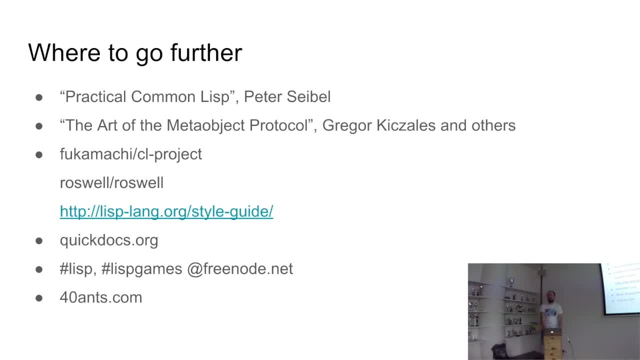 or write a script, And Roswell is actually implementation manager for Common Lisp now, So it's easy to install different implementations and play with them. And yeah, Lisp and Lisp Games are where most Common Lisp developers' lives hang out, at least in the place I'm aware of. 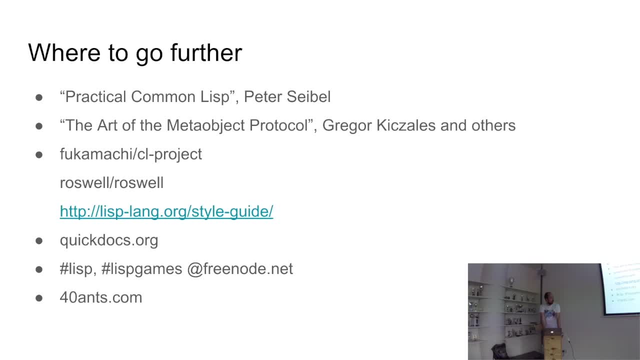 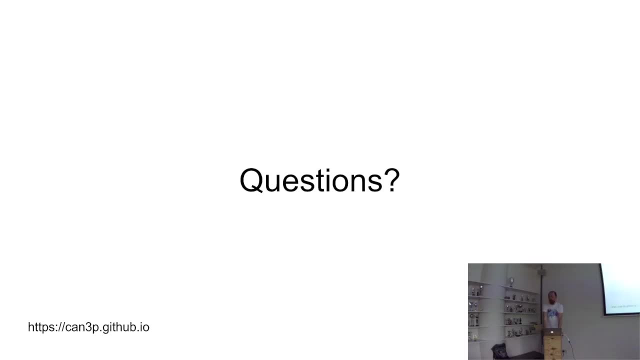 And I'm personally mostly sit on smallcommunity4eonscom. yeah, And this is it. Thank you, I don't know if you have any questions. I have a question. Yeah, So in a couple of slides before, you showed that you can assign value to a function call. 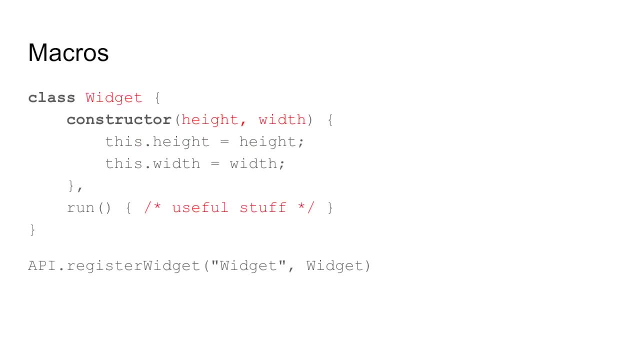 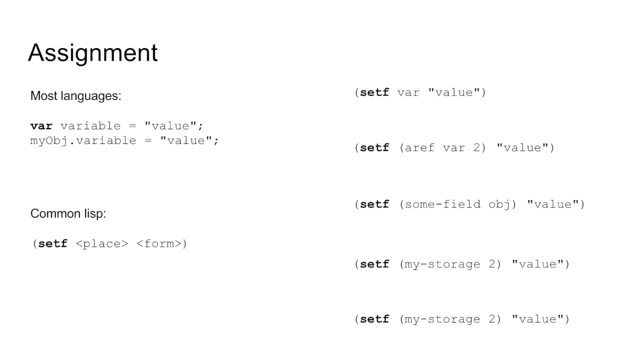 Yeah, What does that do? Yeah, that one like setf, some field object value. Well, basically, there is a protocol of extension for setf. where you can, it can be as simple as defining a function that the name of the function. 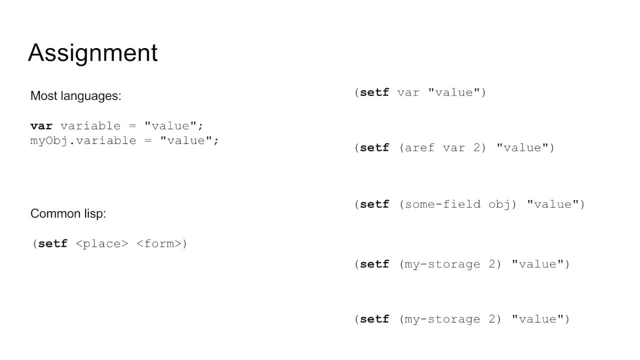 which will be a list, setf, and your name, which will receive the object, I think, and the accessor, like index, for example, and your value, And then it's up to you to place it in a proper place, Right. 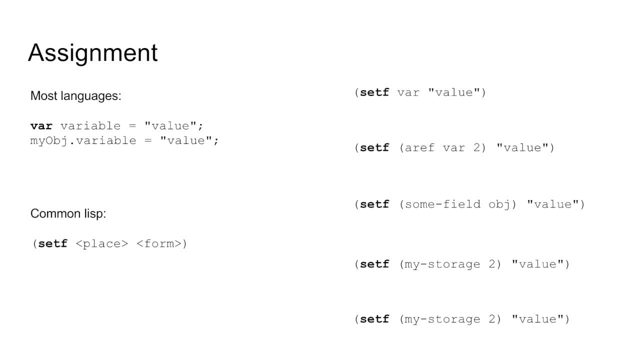 So it's like you define a setter in object, but it's more generic because it's detached from the object, And but this is only one of the options. There is a macro that you can use that is also specified which values it should return. 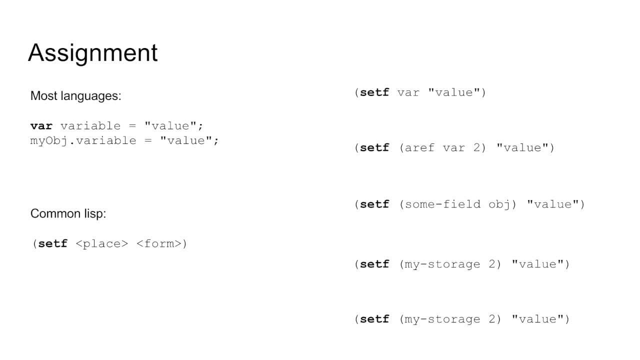 And you can again accepts the argument, some arguments and new values so that you can write the implementation and save it. So it's no magic, it's just an extension protocol. Just a small remark here: in this case, some field is not really a function. 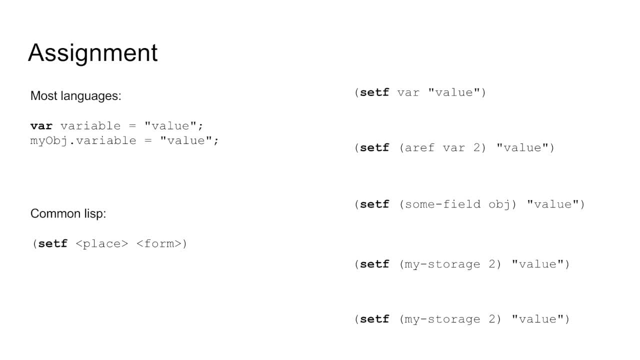 it's a getter of the field of an object. Well, it is a generic function. But the thing is that the setf of the function itself doesn't need to be related to the function. I mean you define the logic You say when you call setf with this function. 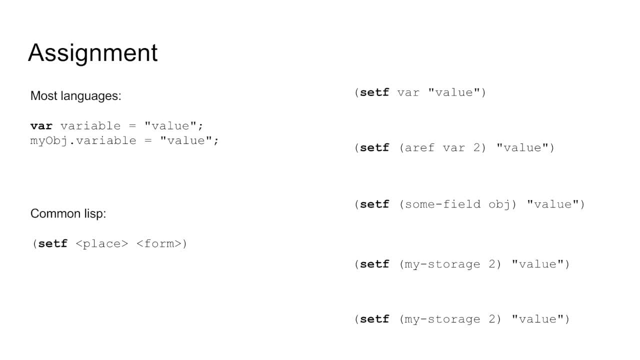 or setf descriptor. you define what you want to do. So you could say, okay, the value will be stored in the database. for example, You define your concept of place. So- and this is a cool part- that you extract away- 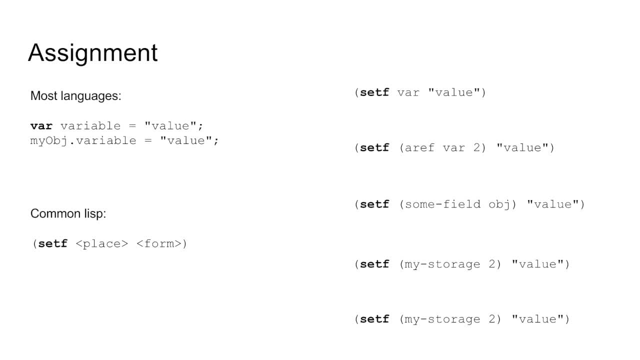 this assignment part and you exactly. you can, for example, write a cache system that will work behind this right Or things like this, And from the client code it will look like an assignment And well, it will work with all the features setf provides. 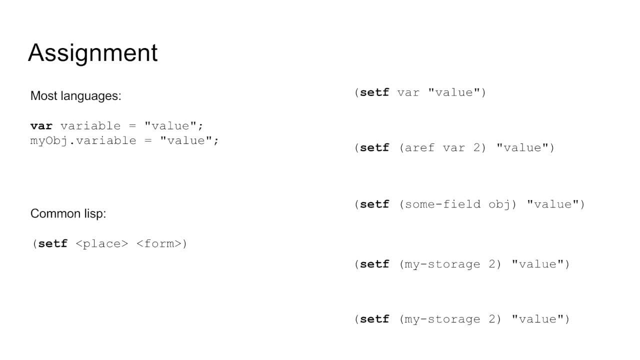 I'd like to. for example, to explain this For someone: in all languages you have the increment operator right And that works with variables and also with accessors. But when you expand it because it doesn't look like a huge benefit, 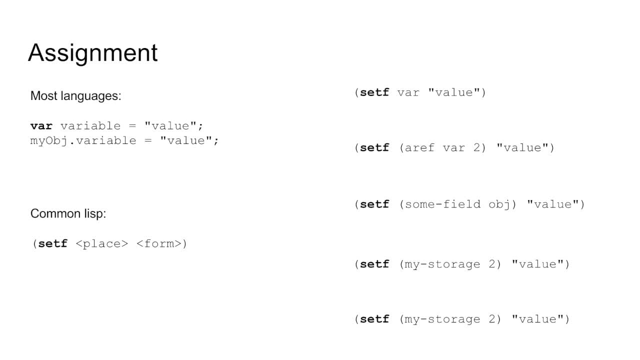 but when you define it with setf, the increment operator will automatically work with your place as well. So if you define a function to say, oh, set a place in the database, you can use incf to increase the value of the database. 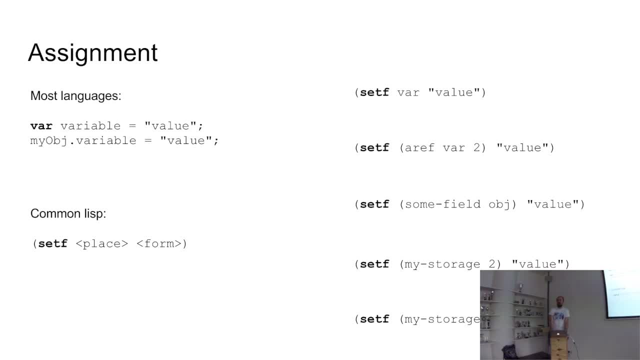 automatically for you. That's what in other languages you cannot do, because the increment operator only works for variable and accessors. Okay, All right, yeah, Yeah. Is there any shell or like REPL-interactive shell that does not suck outside DMAX? 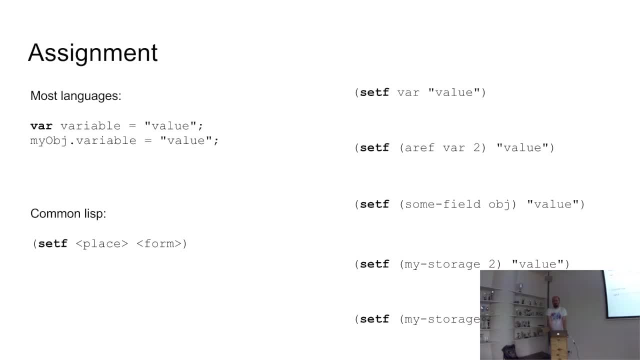 I have no idea. What do you use for the plug-in? I think nowadays there is a Vim replacement for this. Not replacement, but there is a Vim plug-in for this. No, no, no, no, Because a recent version of Vim got the support. 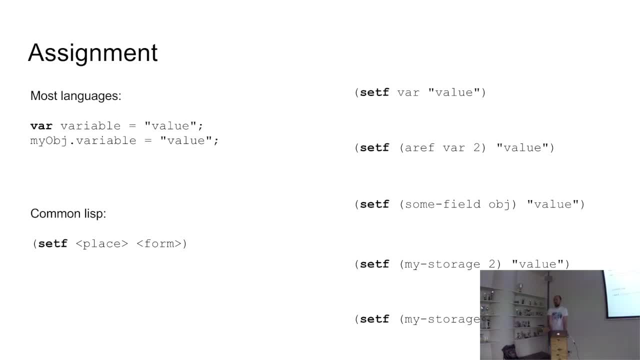 of asynchronous operation, queues and everything. so it became possible to write a slime-like environment, But I don't think that you have a lot of choice. Maybe you can use ListWorks, for example, right, And you will get a Max-like editor. 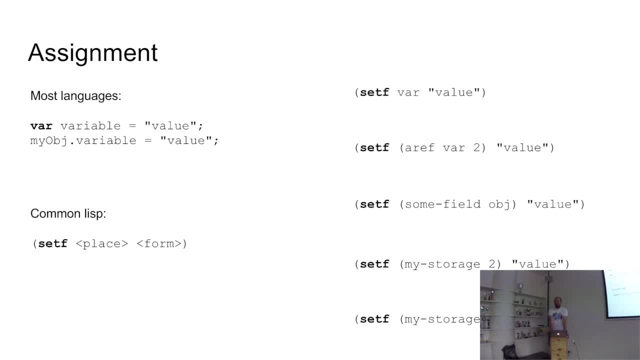 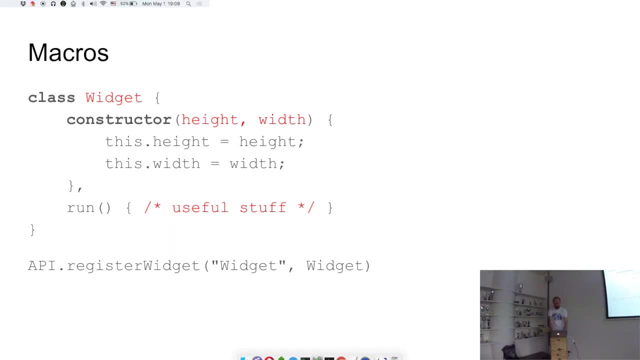 Okay, All right, yeah, Thanks. So No question. No question, Any other questions Cool?